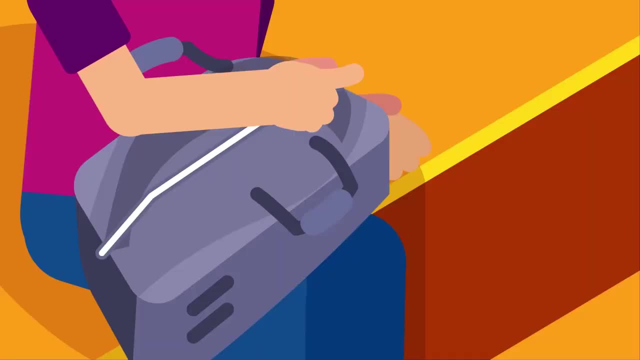 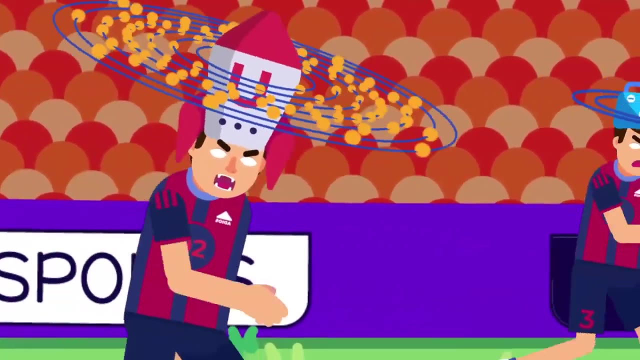 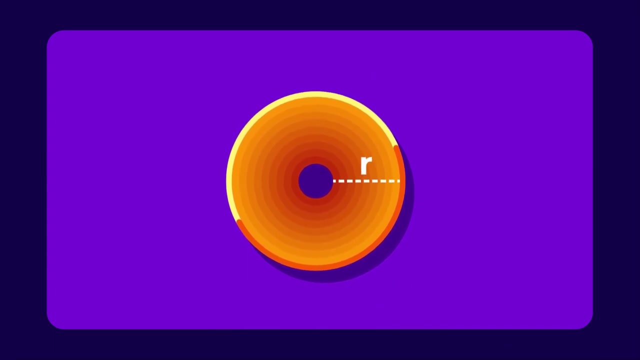 how many electrons you have to spread out between those shells. There are a few patterns, known as trends of the periodic table, that we need to know about. The first trend is atomic radius, which also determines atomic size. An effect of atomic radius is the distance from an atom's nucleus to its outermost orbital, about which 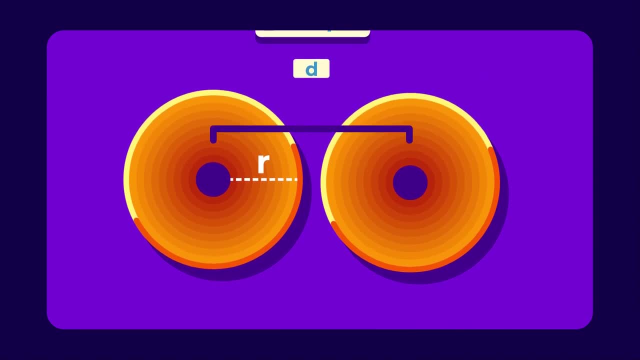 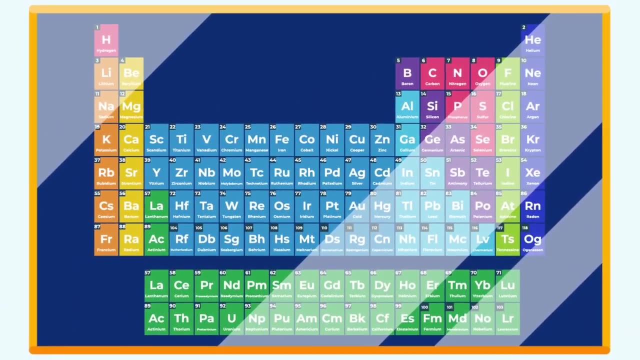 95% of the electron density is found. This can be measured as half of the inter-nuclear distance and it decreases across a period. So as you go from left to right across a period, the atoms get smaller. This is because electrons are being added to. 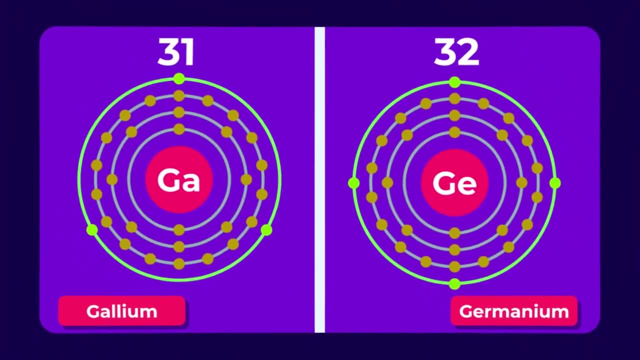 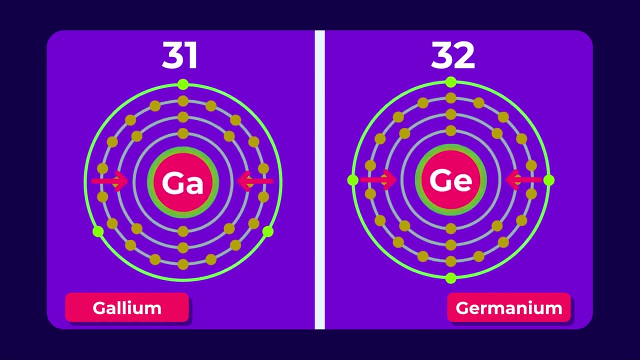 the same shell. Why does this matter? Well, the outer shell electrons are being pulled inwards by the positive protons in the atom's nucleus. So the more electrons on the outer shell, the stronger the attraction, which means the more inwards the atom will be pulled. 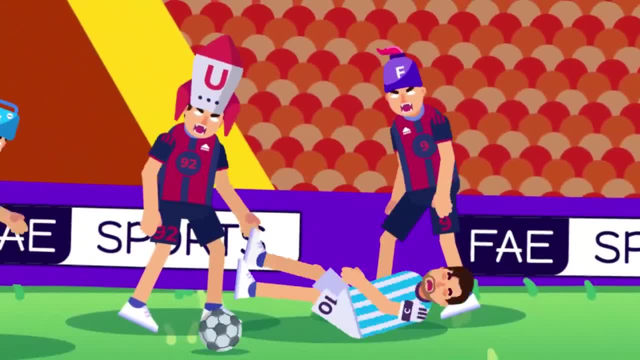 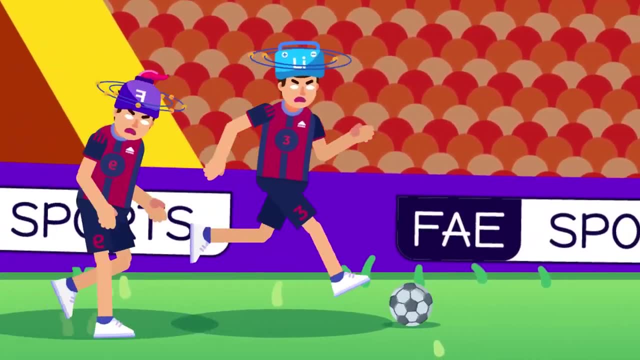 in, So the smaller it'll be. This attraction pulling the electrons inwards is called the electromagnetic attraction. The next trend is ionic radius, which is the radius as atoms form ionic bonds. It generally decreases as you go across a period of time. The second trend is ionic radius, which is 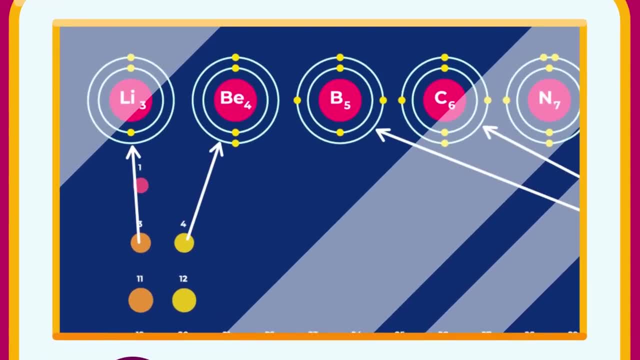 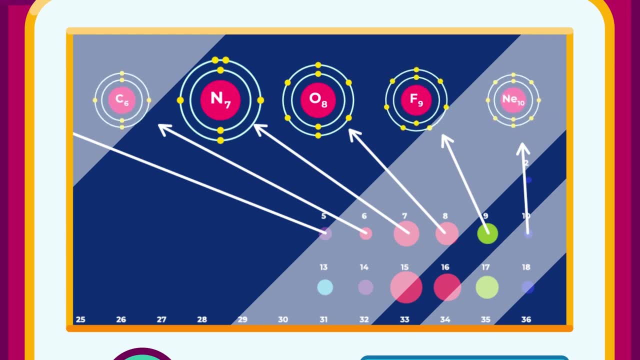 to go across a period from left to right. This is because there are more protons in the atoms, but with the same number of shells, And so the electrons on the outer shells are subjected to electromagnetic pull, pulling them inwards, While forming bonds, cations. 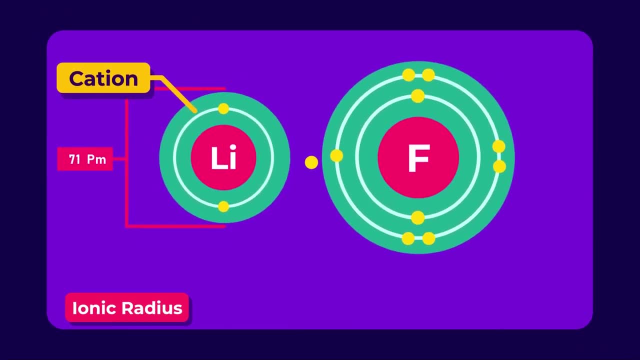 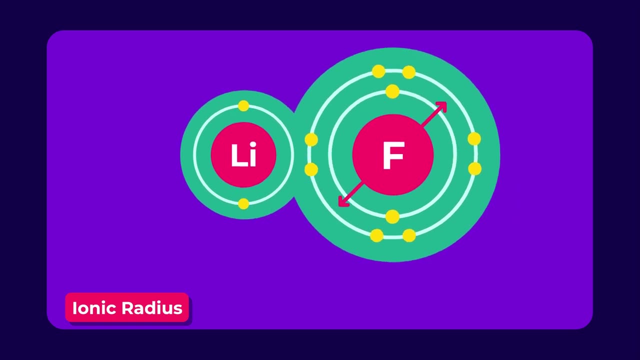 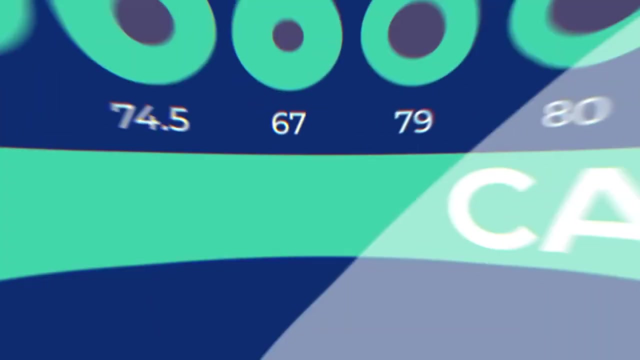 are smaller than its parent atoms as electrons are removed from the outer shell. Anions are therefore larger than the parent atoms as electrons are added to the shell, resulting in increased repulsions between electrons and a decreased electromagnetic attraction numbered by electrons. This makes the trend a bit complex. Knowing about the atomic radius and ionic radius is 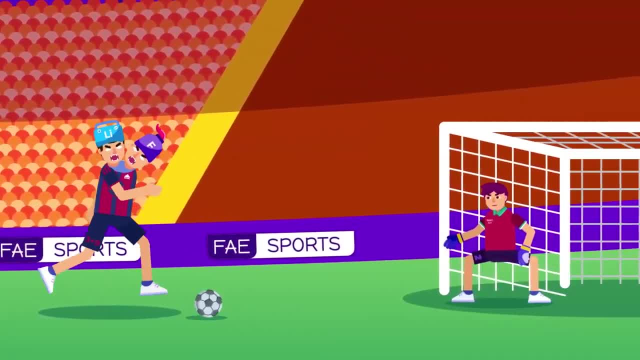 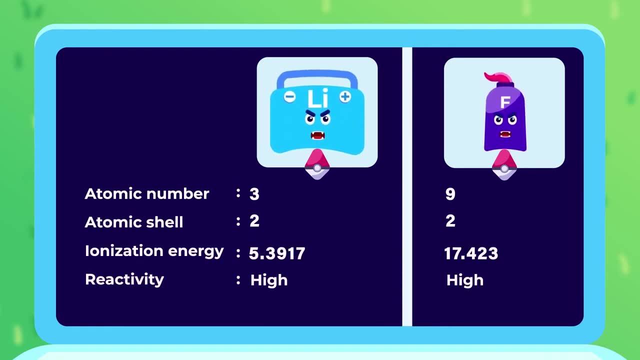 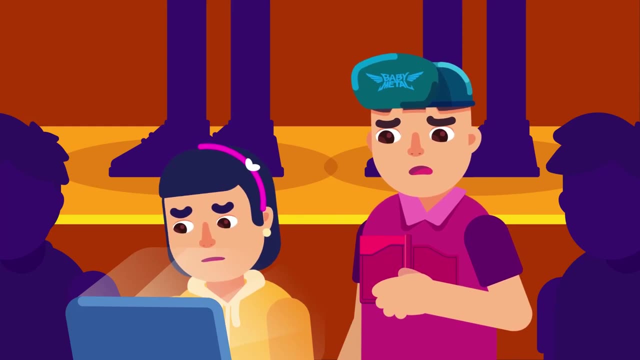 very important. It not only gives the information about electron distribution, but also helps us explain the behavior of atoms of an element such as energy and reactivity. However, being informed about trends in radius is not enough to understand the periodic table thoroughly, So in the next video we will dig deeper into other trends in periods: Ionization, energy. relativity and lastly, electronegativity.